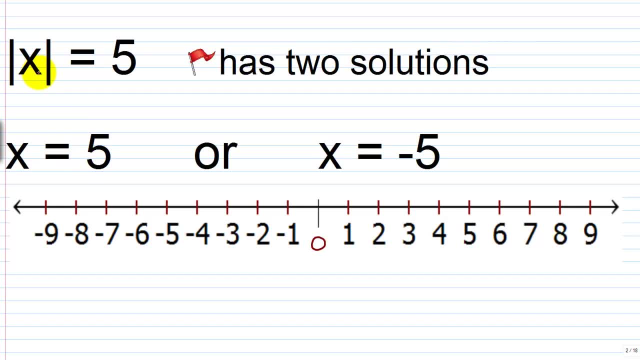 And you would get an absolute value of 5.. Absolute value of 5 is 5. And then negative 5 can be plugged in for x. Remember, if you have a negative value, you plug it into the absolute value operation. it makes it positive. 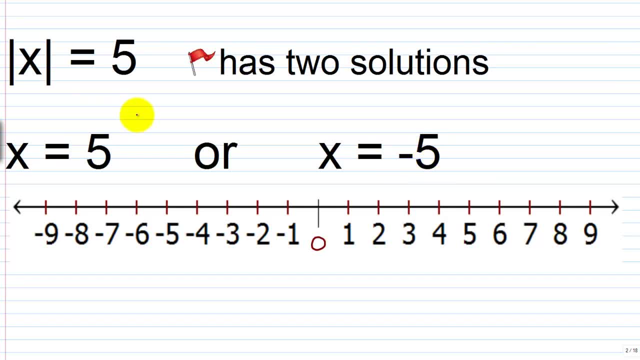 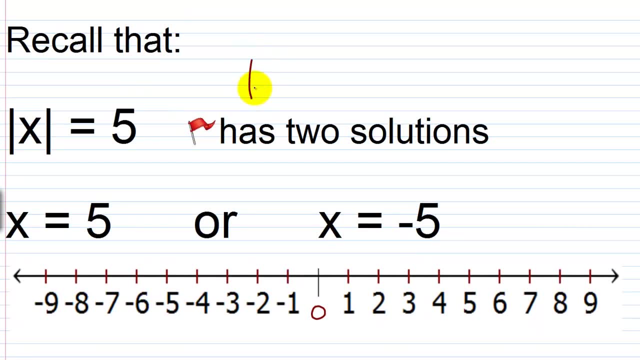 So the absolute value of negative 5. 5 will be 5 as well. So when you get a simple absolute value equation like this, you basically have this or scenario. So if I had absolute value of x equals 9, it would just be x equals 9.. 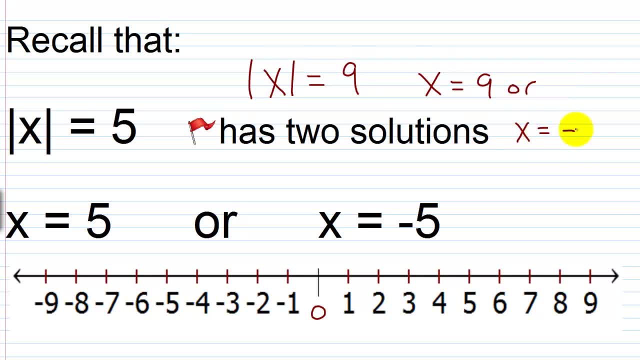 Or x could be negative 9.. x could be negative 9. Because if I plug either of those in for x, I take the absolute value of them. I get a result of 9.. So now that you understand that, let's kind of move into the next step. 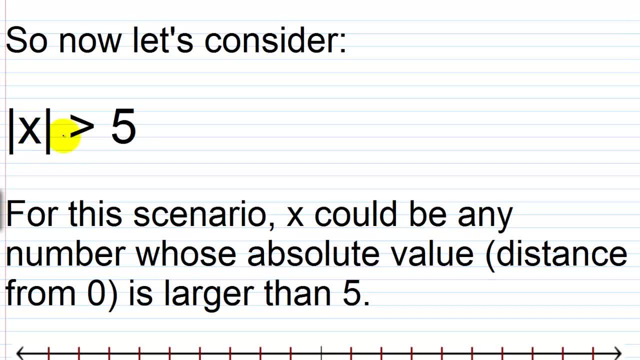 Which is to consider something like this, Where we have the absolute value of x is greater than 5.. So now we're not dealing with, you know, one or two values here. We're dealing with a range of values, Because this is saying: give me all the numbers whose absolute value is greater than 5.. 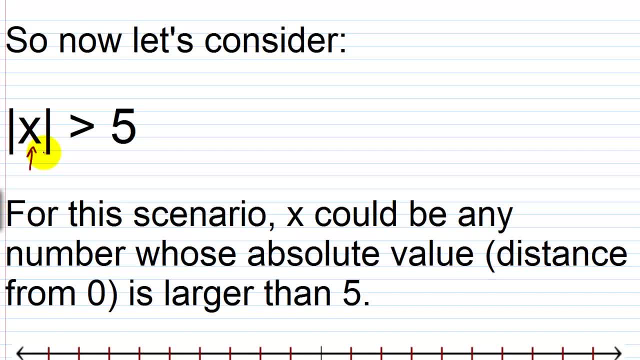 Whose distance from 0 on the number line is larger than 5.. Well, if we think about this, we know that x could be greater than 5.. We always do kind of the positive example: first You just remove the bars and you have x is greater than 5.. 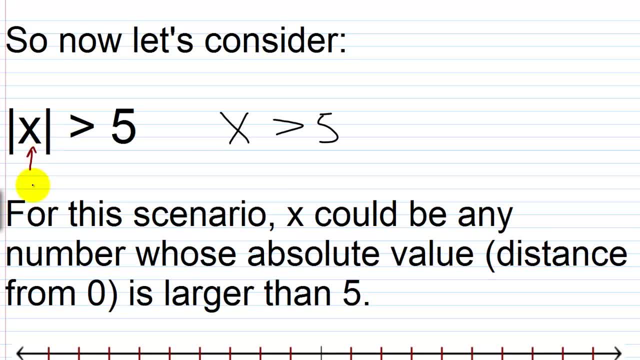 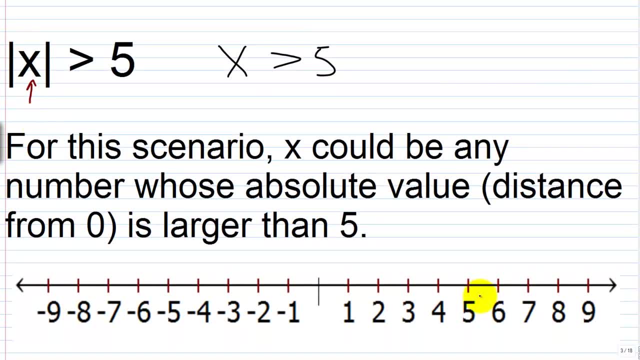 Because if I plug in something like 6 or 7 or 8, I take the absolute value of it. I'll get 6 or 7 or 8. And that's all larger than 5.. So any number that you can think of- just kind of looking on the number line here- larger than 5 would work. 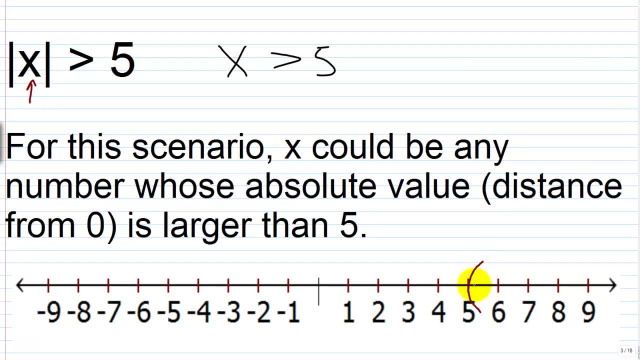 So I would just put a parenthesis at 5 to say that's not included And just shade everything to the right. We also have to consider negatives, Negative values as well, because, remember, if I plug something negative into the absolute value operation, it makes it positive. 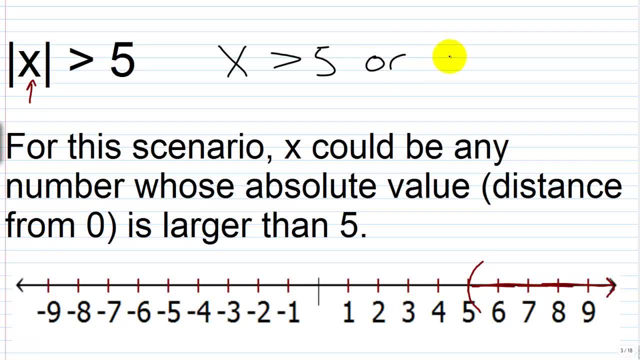 So it also means that the negative we could say, or the negative of x, could also be greater than 5.. Because if I think about numbers that are smaller than negative 5, moving to the left, bigger negatives, smaller numbers, So something like negative 6.. 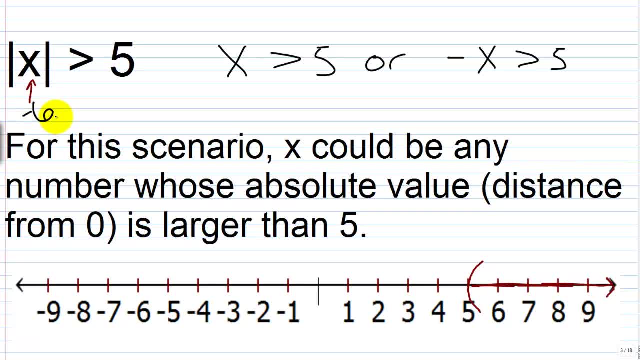 If I plug a negative 6 in there and I take the absolute value of it, it's going to be larger than 5.. Because the absolute value of negative 6 is 6.. 6 is larger than 5.. So anything to the left of negative 5 would work as well. 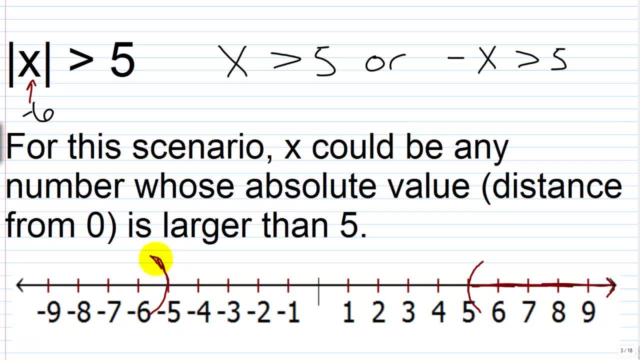 So I'd put a parenthesis at negative 5.. That's not included. That's a bad parenthesis. Let me kind of redraw that And I'd shade everything to the left because all of this would work Now. typically, when you first see these examples in your textbook, you're not going to see negative x is greater than 5.. 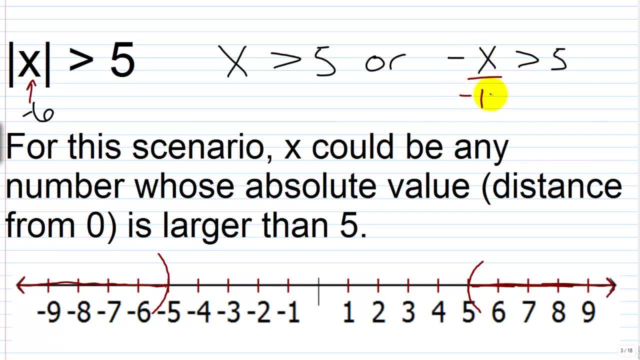 And the reason for that is they divide Each side by negative 1, or they multiply by negative 1,. however, you want to think about this And this is going to get flipped right, So what you'll have is: let's just erase this, flip this sign. 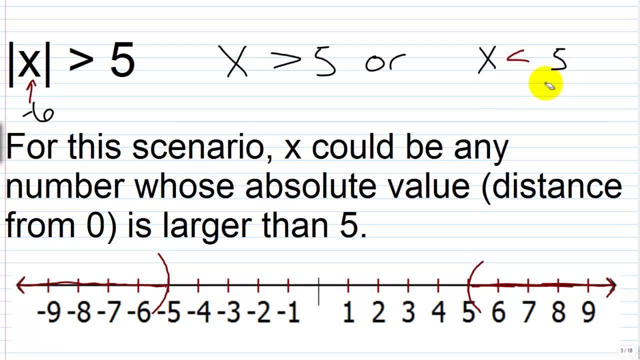 This will be less than. and then 5 divided by negative 1 is negative 5.. So you'll see x is greater than 5 or x is less than negative 5.. So the sign gets flipped and then this becomes negative. And you're going to hear me say that over and over again, because it's the easy way to remember it. 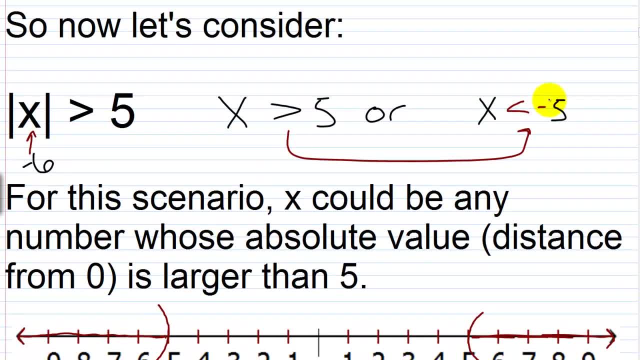 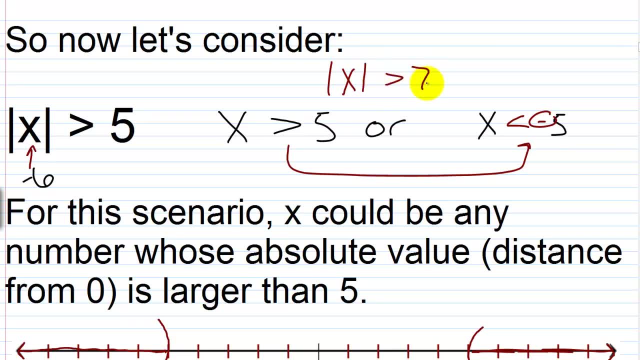 Sign gets flipped. Sign gets flipped, This becomes negative. So if I had something like absolute value of x is greater than 7, you would have what You'd have: x is greater than 7 or x is less than negative 7.. 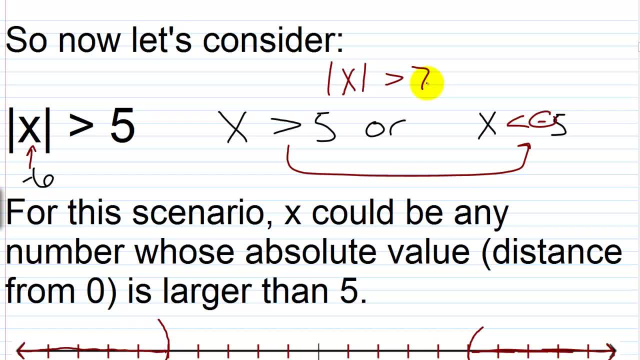 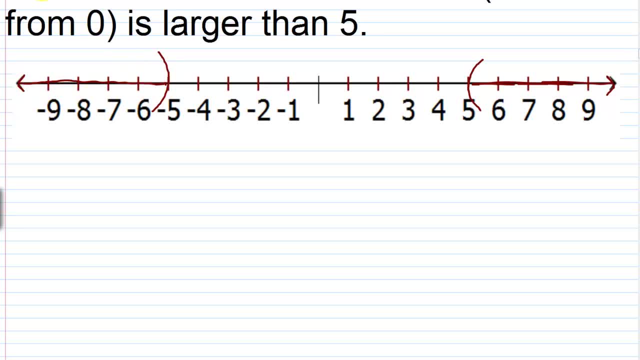 Now the last thing I want to do is kind of show you how to write this in interval notation And you're going to have the union of two sets right. So basically you would have kind of this first set here which is coming from negative infinity. 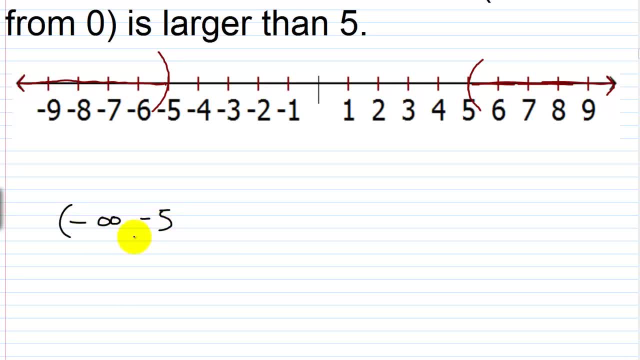 And it goes up to, but does not include negative 5.. And it's the union of this with this other set over here, which doesn't include 5 but anything greater, going out to infinity. So that's how you would use interval notation to write your solution. 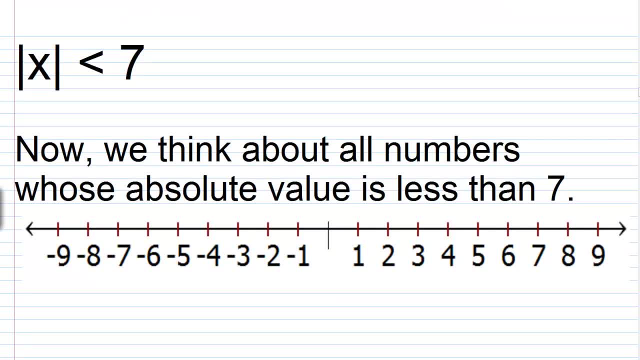 Okay, now the other scenario that we come across is the less than We looked at greater than Now we're looking at less than. So we have: the absolute value of x is less than 7.. So now we think about all numbers whose absolute value, or distance from 0, is less than 7.. 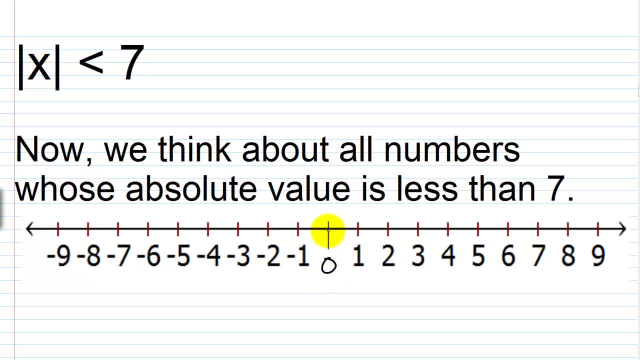 So if I look at kind of starting at 0,. well, I can kind of go out this way, because this would have a distance of less than 7,, less than 7,, less than 7, up to, but not including 7, right. 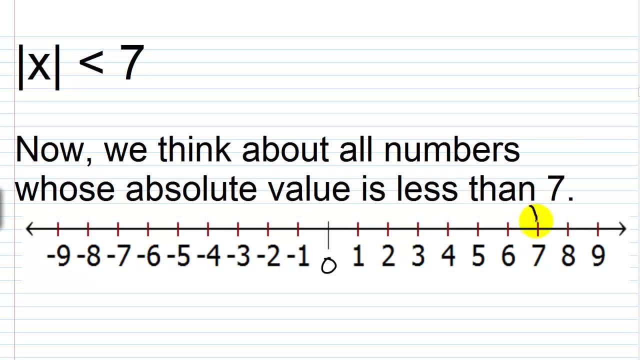 7 would not be included because 7 has an absolute value of 7.. So I can't include that. I'm going to put a parenthesis there And I would shade everything And I'm going to stop at 0 for right now. 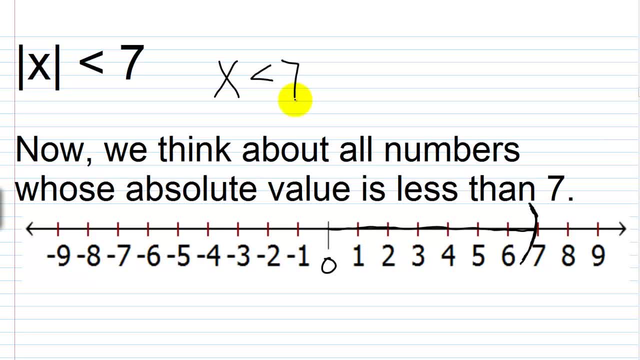 Because I know that x could be less than 7.. But there's another scenario, because we also have negative values that we can plug into the absolute value operation, It could also stay that, and the opposite of x or the negative of x could also be less than 7.. 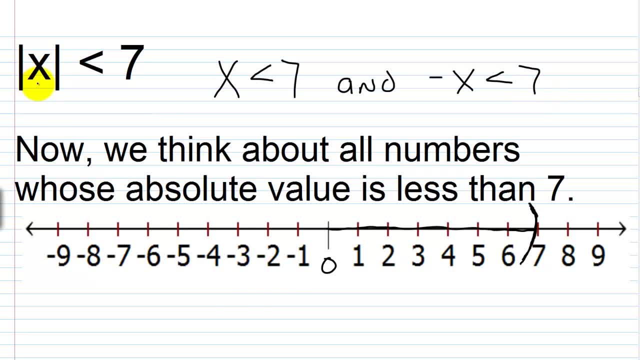 Because if I plug in something like negative 3,, negative 3, take the absolute value of that, you get 3.. 3 is less than 7.. That works out. So this would go to the left until we get to negative 3.. 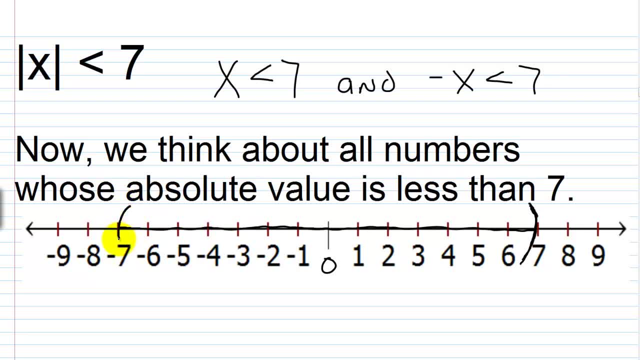 We'd put a parenthesis there because negative 7 couldn't be included. because if I put a negative 7 in there, take the absolute value of it, I get 7. And 7 is not less than 7, right, It would only work if we had a, you know, a non-strict inequality like that. 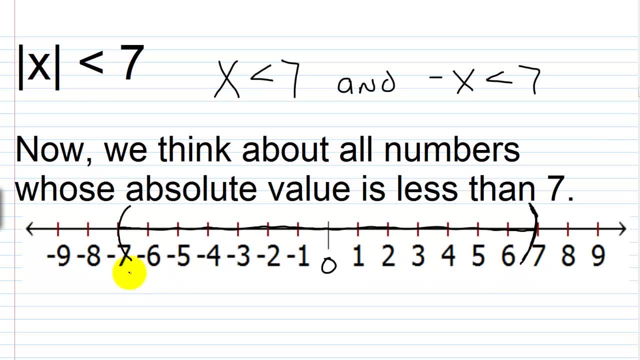 But we don't have that here. So graphically, this would be your solution, right? It could be anything between negative 7 and 7.. All those numbers would work And we end up with this inequality here, And again, I can just divide that. 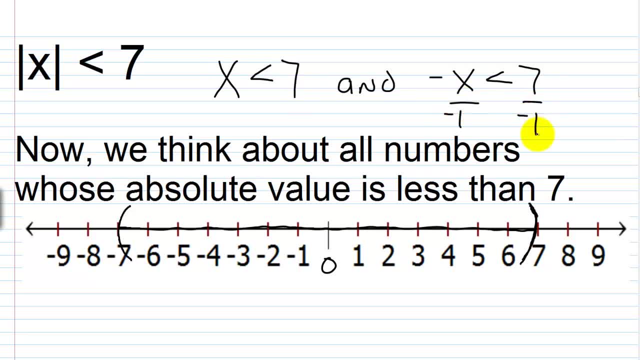 Again, I can just divide both sides over here by negative 1.. And this has to flip. So what will I get? I'll get: x is greater than greater than negative 7, okay, Negative 7.. And it's common to see this written as a three-part inequality. 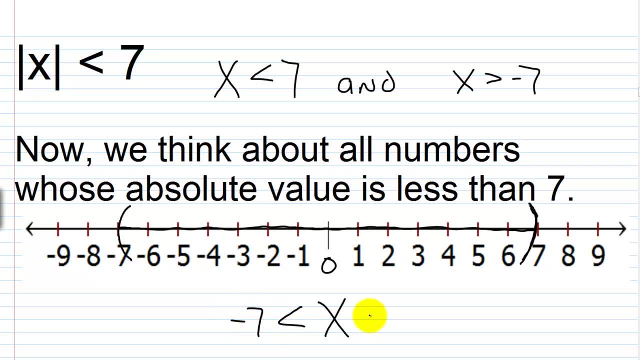 You'll have x in the middle and it's greater than negative 7 and it's less than 7, okay, Or you can write it like this. We've already talked about compound inequalities. It has to satisfy both. It has to be greater than negative 7 and less than 7.. 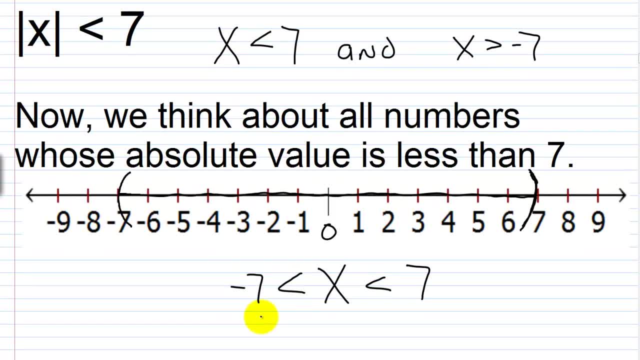 So that's what we have in this scenario, here, And an interval notation just looks like this: Negative, 7 to 7, right, And there's a parenthesis at each because neither are going to be included, All right. So these are very simple problems and the ones that you're going to see at the beginning of the chapter. 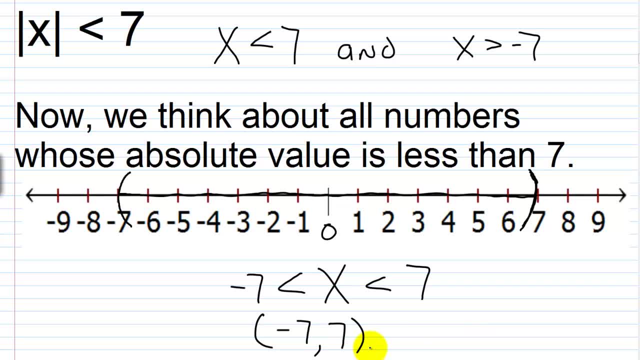 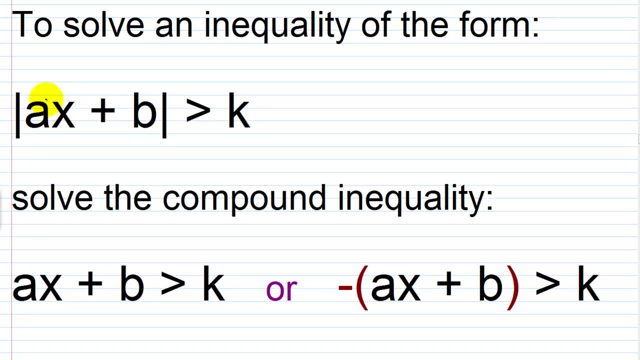 But you're going to get harder stuff. Now let's take a look at how to solve those type of problems now. Okay, So to solve an inequality of the form. And we have this: ax plus b inside of absolute value bars is greater than k. 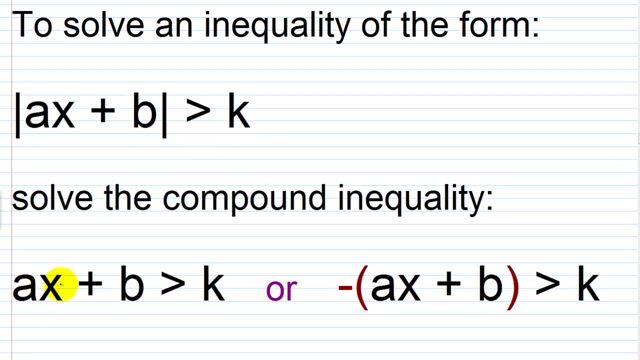 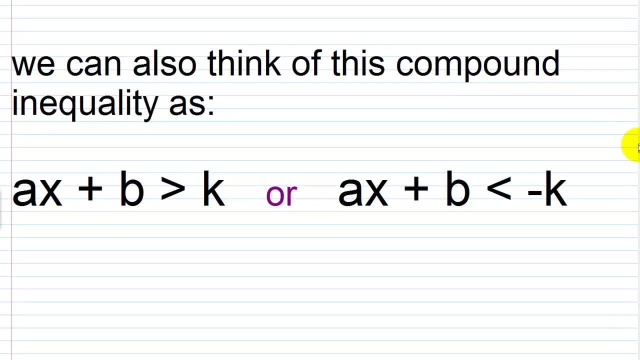 We're going to solve the compound inequality- Ax plus b is greater than k- or the negative of this whole thing: ax plus b is greater than k. Now, what I'm going to do is I'm going to write this differently And I have that down here already. 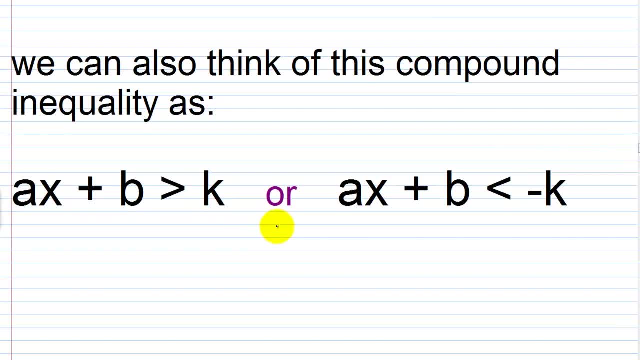 We can also think of this compound inequality, as ax plus b is greater than k, or ax plus b is less than the negative of k. All we did was we divided both sides by a negative, So this got flipped and this became negative. That's it. 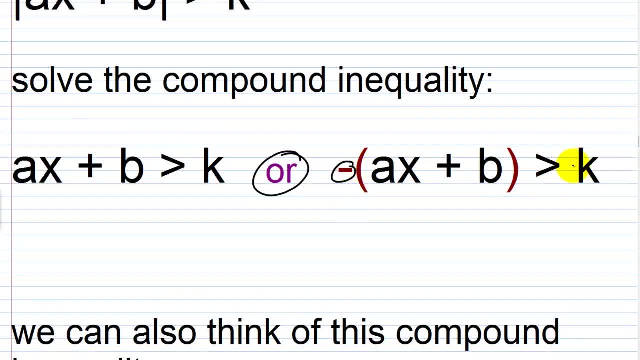 Just kind of scroll back up so you can see this Here: this is negative and this is positive And this sign is a greater than. So if we divide both sides by negative 1,, basically, this is going to cancel, This will become less than and this will become negative k. 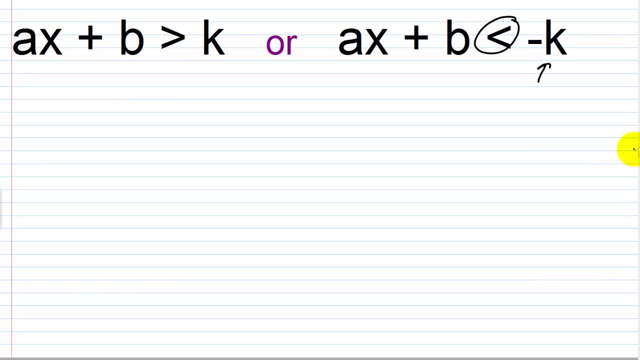 Which is what we have down here. So it's always going to be an or scenario when you start off with greater than Okay. But here's what I want to tell you so that you remember this: You have your first scenario where you just kind of remove your bars. 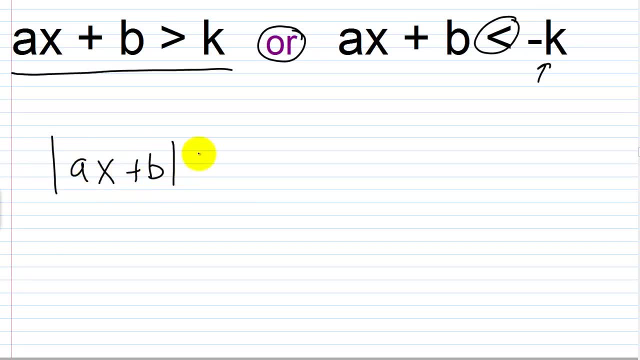 You have absolute value of ax plus b is greater than k. Just remove those bars and you get this right here. Then you remember, because it's greater than you're going to have the or statement Okay, And you're going to end up with the second one here. 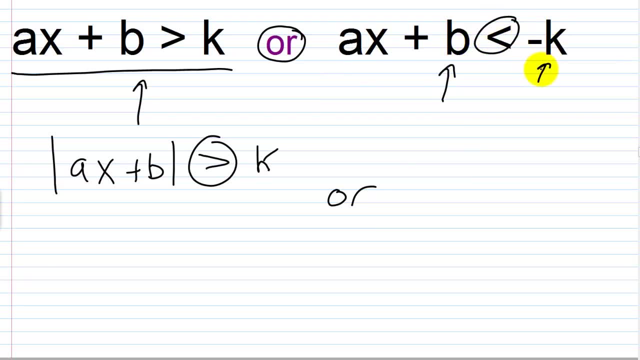 Remove the bars. You're going to flip this. make this negative. Flip this, make this negative. Okay, So you have ax, Ax plus b is greater than k or ax plus b. Flip it. Flip that. Make it negative. 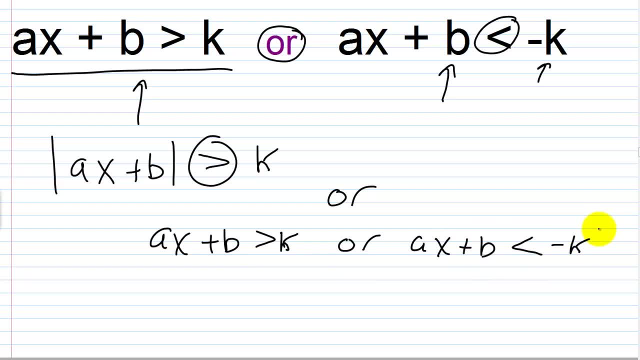 Negative k. And again, I know I say this all the time. When we work with abstract stuff, it's kind of hard to figure out what's going on. Once you get into some examples and you practice enough, this really does become pretty easy. 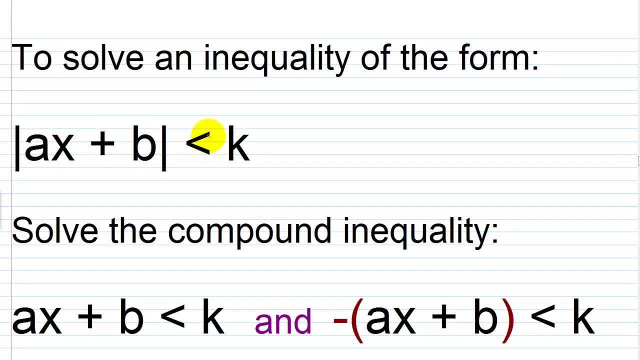 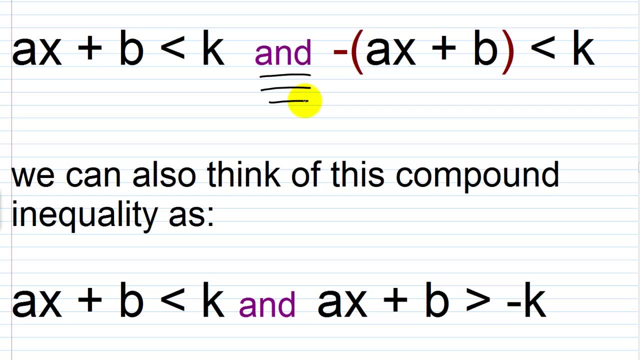 All right. So the other scenario is to solve an inequality of this form where we have a less than Okay, So the absolute value of ax plus b is less than k, And for this we solve the compound inequality We have: ax plus b is less than k, and so notice how we're using and here 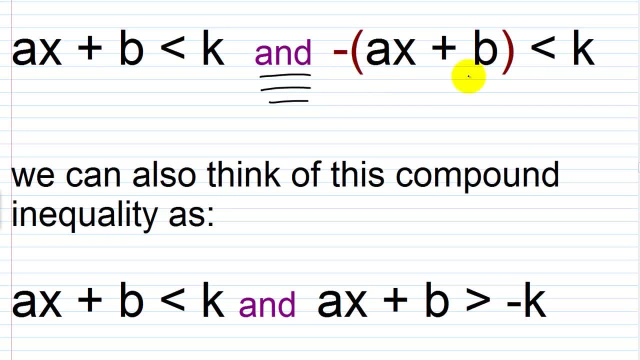 The negative of this ax plus b is less than k. Again, I can divide both sides here by negative 1. This will get flipped and this will become negative k. So in other words, let me kind of erase this. I'll show you that what happens down here. 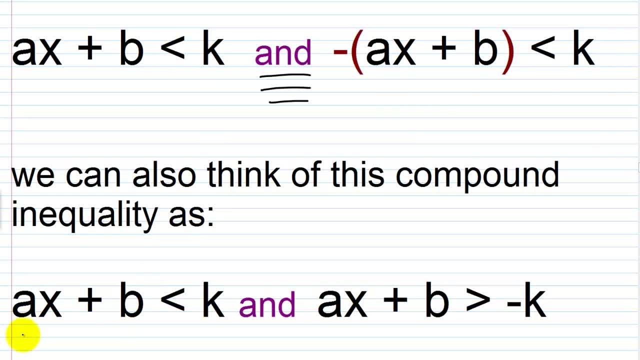 You have: ax plus b is less than k. So that's the first scenario. Just remove your bars. and your second scenario is essentially: this part is the same ax plus b. You're going to flip this. All right, This is getting flipped, and then this becomes negative. 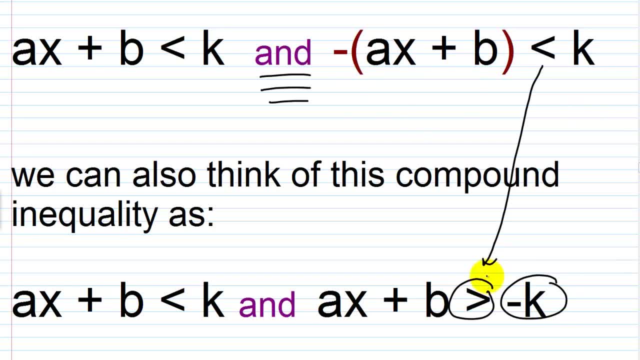 And that's just because we divided again both sides by negative 1.. So this gets flipped and then this becomes negative. So the main thing to remember is that if you have a less than it's an and statement, If you have a greater than it's an or statement. 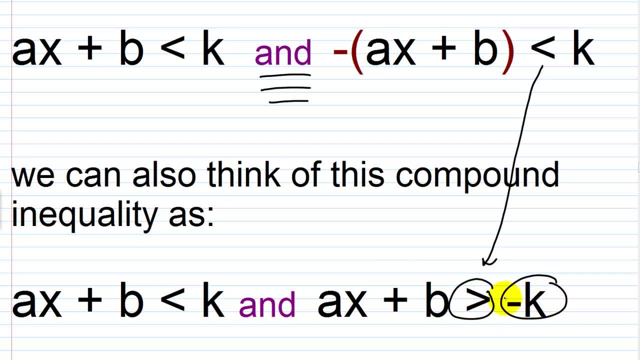 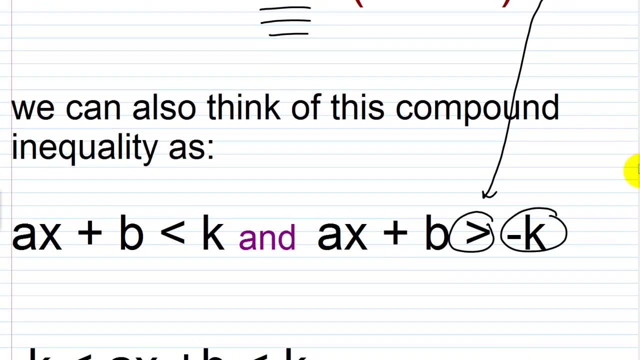 This part is always the same. You flip the sign. Flip the sign, Make it negative. So remove the bars. Flip the sign, Make it negative. And then the first setup is kind of just remove the bars. And here it shows you that you can basically just write this as a three-part inequality: 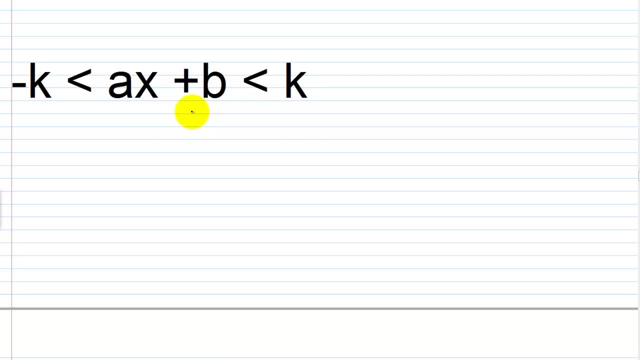 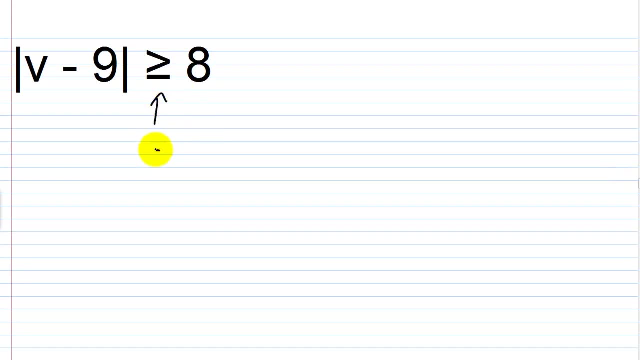 where ax plus b is going to be greater than negative k and less than k. Let's take a look at kind of an easy one And we'll want to note here that we have a greater than symbol. I know it's a greater than or equal to, but we're just going to say it's greater than. 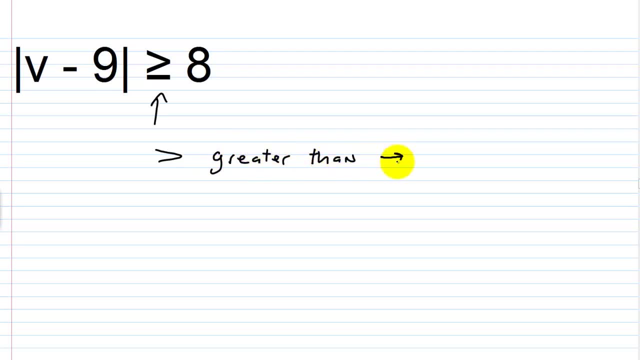 It's greater than. So we know this is an or statement. That's what you have to memorize. So the first scenario here we have: the absolute value of v minus 9 is greater than or equal to 8.. Just remove the bars. 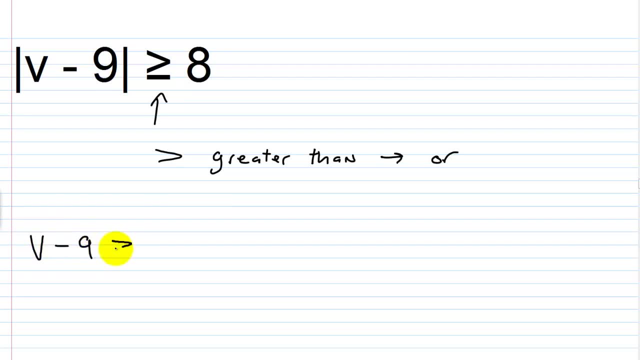 Just remove the bars, So we'll have v minus 9 is greater than or equal to 8.. That's your first scenario. Then, or The second scenario: remove the bars, So v minus 9.. Flip the sign, So the sign will now be less than or equal to. 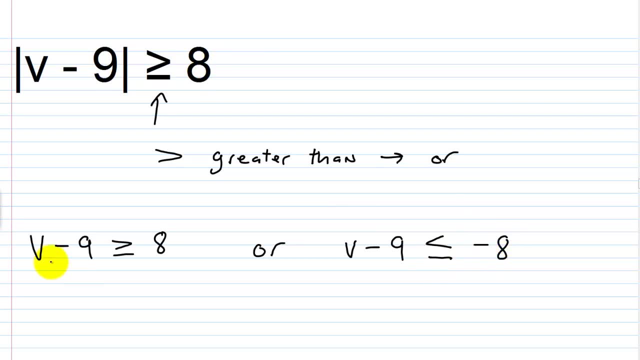 And then make this negative, Negative, 8.. So the first one: you just remove the bars, Then you have your, or Then you have basically v minus 9.. Flip the sign, Make it negative. Let me write that Flip. 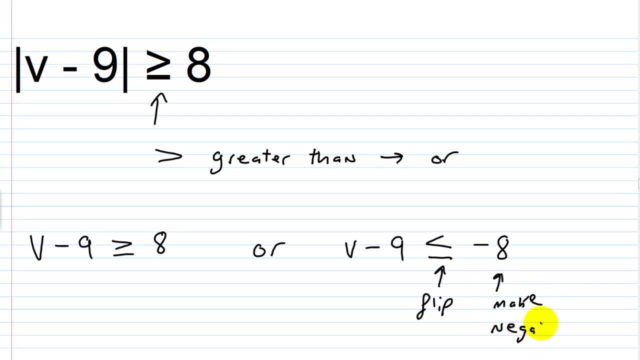 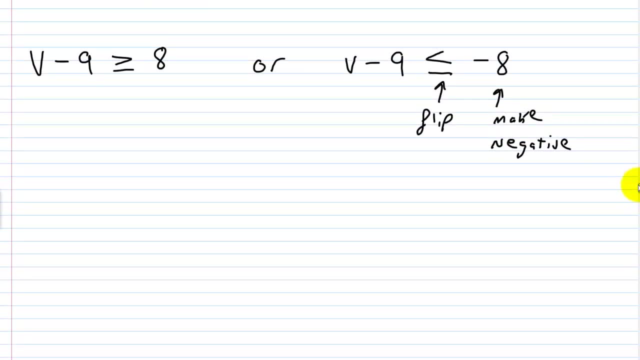 Make Negative. And again, once you start doing this a lot, you just remember it. You just need to practice enough. So let's solve this one here. This v minus 9 is greater than or equal to 8. I just add 9 to each side. 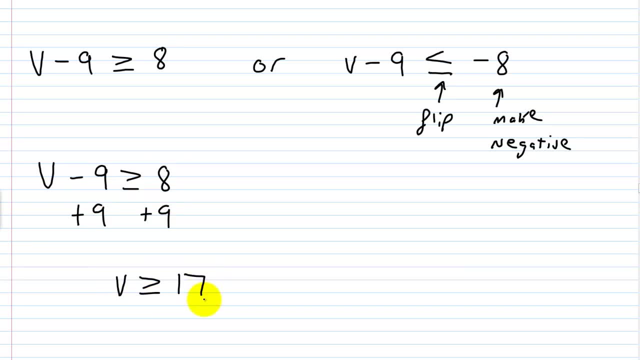 And I'm going to get v is greater than or equal to 17.. And then over here I have v minus 9 is less than or equal to negative 8.. I add 9 to each side. I'm going to get v is less than or equal to 1.. 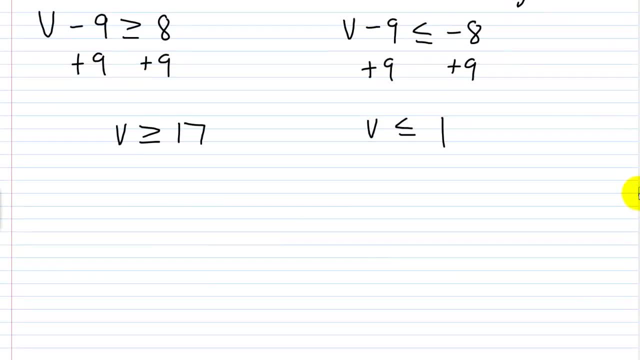 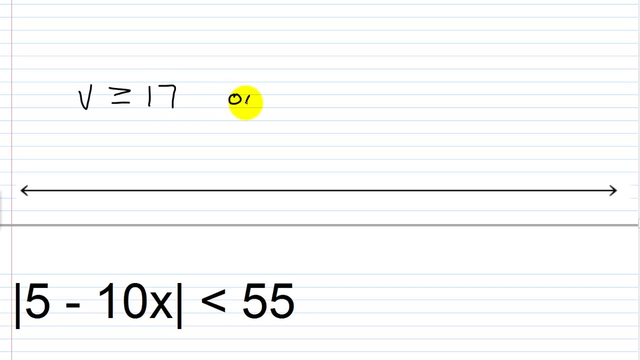 So let's bring these two solutions down to the number line, So we can have: v is greater than or equal to 17.. Or v can be less than or equal to the number 1.. So using kind of interval notation, if v can be less than or equal to 1,. 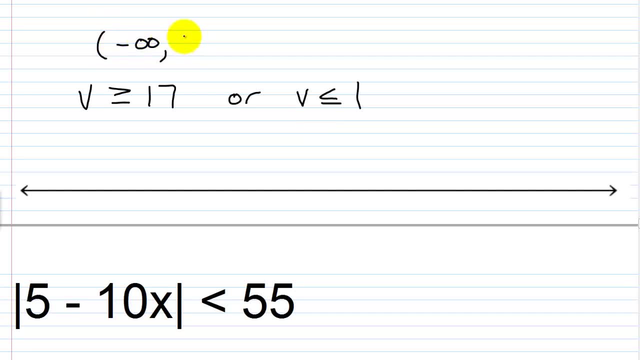 you'll be coming from negative infinity up to and including 1.. And it's the union of this with this right. here v can be greater than or equal to 17.. So it includes 17 and then anything larger. So I have a blank number line here, because my normal number line just goes from negative 9 to 9.. 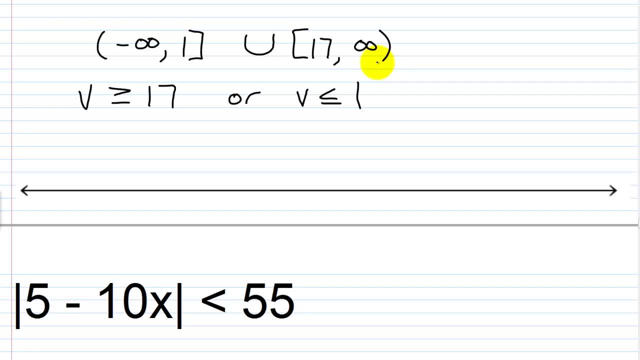 So I have a blank number line here because my normal number line just goes from negative 9 to 9.. So I have a blank number line here because my normal number line just goes from negative 9 to 9.. And I want to note that let's say 0 is right here. 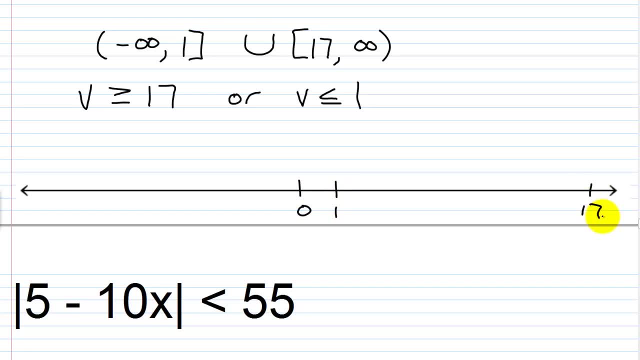 Let's say 1 is here And I don't know. let's say 17 is somewhere over here. So if it's anything larger than 17 or equal to 17,, I'll put a bracket at 17 and just shade everything to the right. 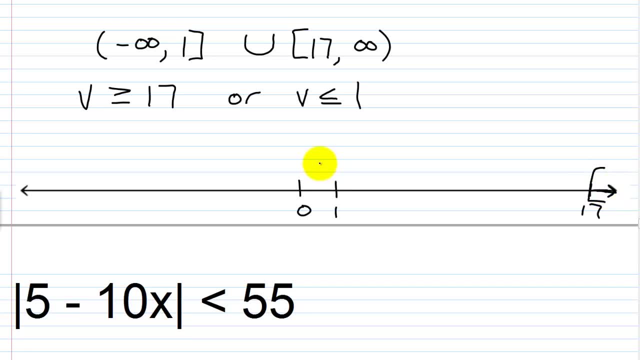 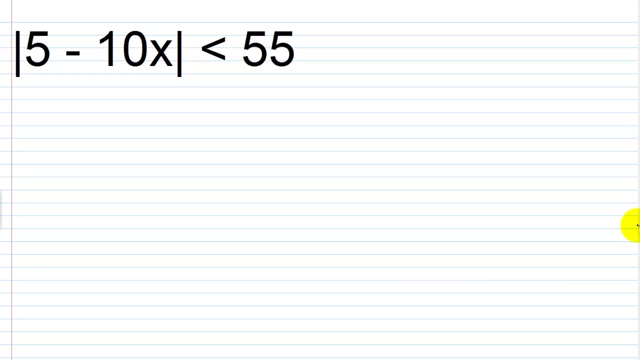 And then, if it's anything including 1 or less, I'll put a bracket at 1 and shade everything to the left. Shade all of this to the left, And that would be your solution set graphically. Okay. so for the next one, we have the absolute value of 5 minus 10x is less than 55.. 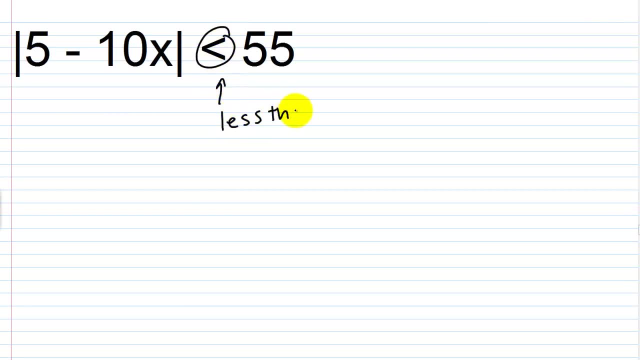 So we have a less than now, Less than- And this gives me an and Greater than gives me an, or Less than gives me an, and That's what you need to remember. So the first setup is to remove the bars, So everything will just look like this right now. 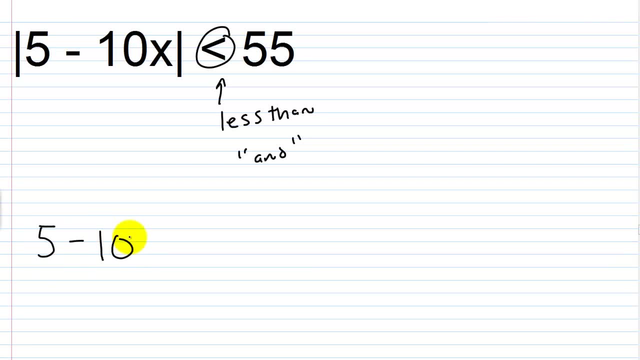 But you're just going to remove the bars, So 5 minus 10x is less than 55.. So then, and Your second setup is to remove the bars, So 5 minus 10x. Flip the sign. Flip the sign. 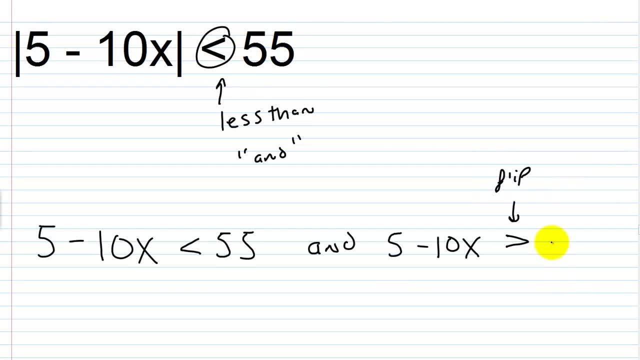 Flip And then make this negative. So instead of 55, it's negative 55. And just say: make negative All right, And we can put this together as a three-part inequality if we want. I know it's usually easier for me to solve it like that. 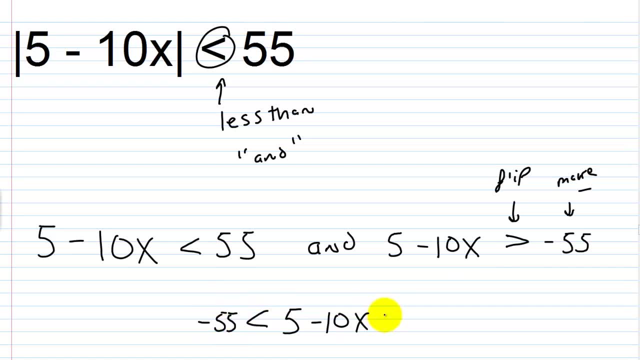 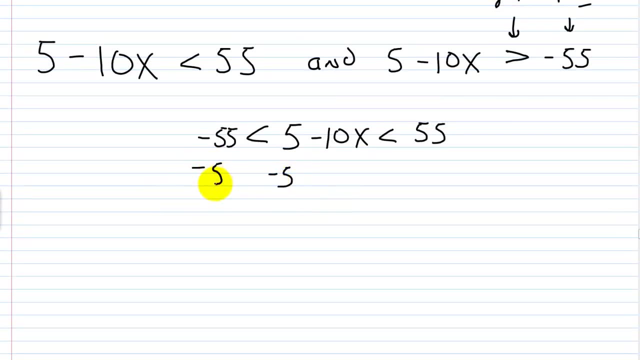 So it's greater than negative 55.. And it's less than positive 55.. Let's see what we get when we solve this. Let's subtract 5 away from each part, So this will become negative. 60 is less than negative 10x. 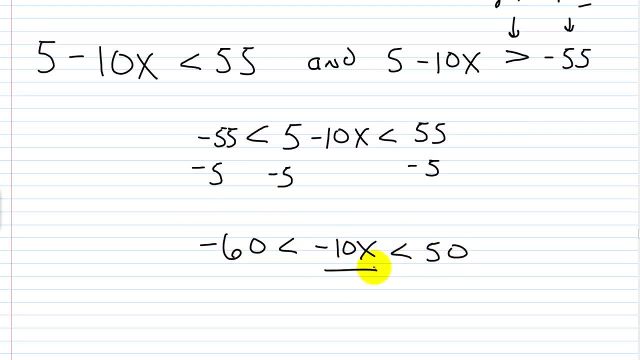 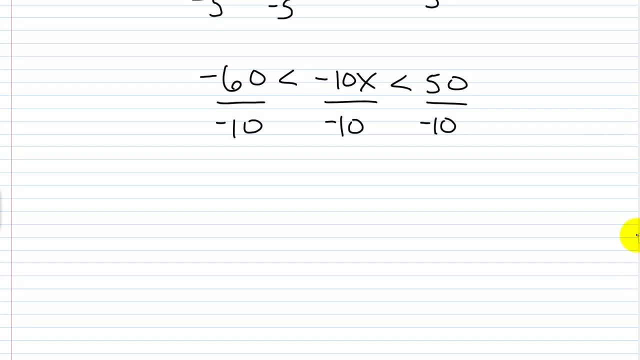 Which is less than 50.. We'll divide each part by negative 10.. And remember, because you're dividing by a negative, you have to flip the direction of the signs. So negative 60 divided by negative 10 is 6.. 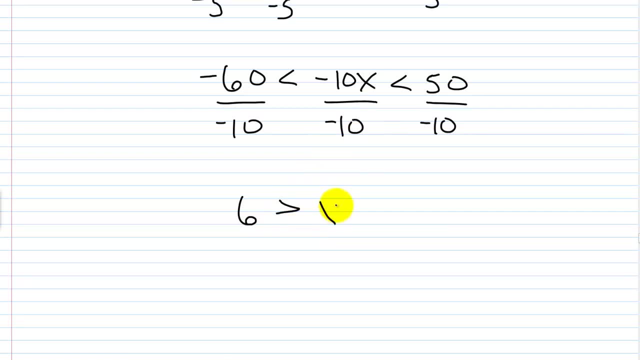 So you'll get 6.. This will become greater than This will be x. This will be greater than 50. divided by negative 10 is negative 5. And we'll rewrite this in terms of the number line. So negative 5 is less than x, which is less than 6.. 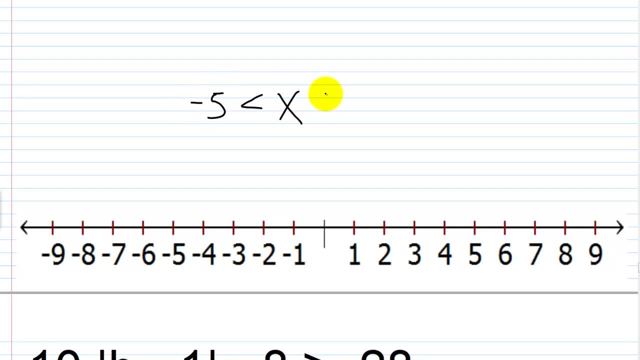 So again, x is going to be greater than negative 5 and less than 6.. An interval notation: This is the numbers between negative 5 and 6. And they're not included, So you make sure you use a parenthesis in each. 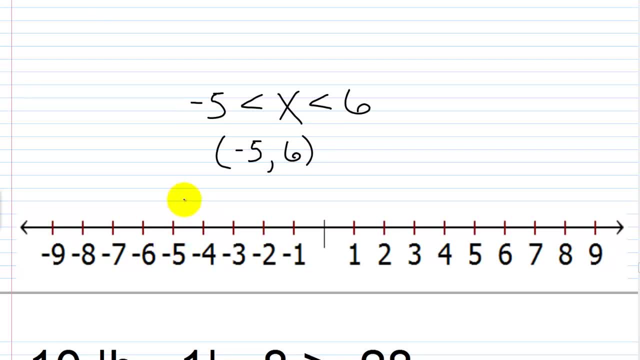 And then graphically, here's negative 5. It's not included, Here's 6. It's not included. And I want to shade all of this in between, Because anything in between negative 5 and 6 will work as a solution. 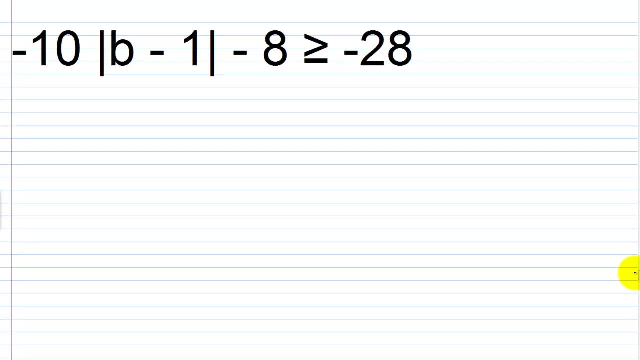 Okay, let's take a look at a harder problem And basically what we need to understand here. we have negative 10 times the absolute value of b minus 1 minus 8 is greater than or equal to negative 20.. We want to isolate this absolute value part right here. 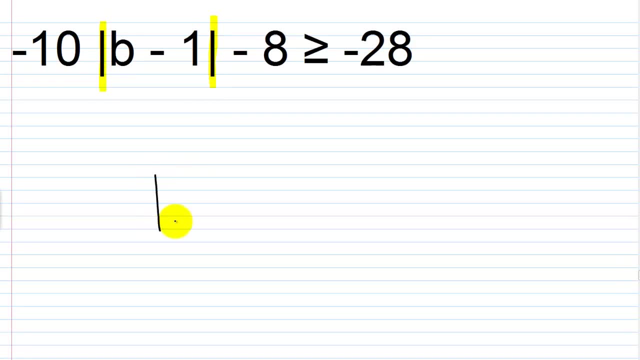 Okay, that's what we do to start, Because we want something that looks like this: This absolute value of ax plus b is greater than k, Or this could be less than k, whatever. Basically, we want the absolute value operation on one side. 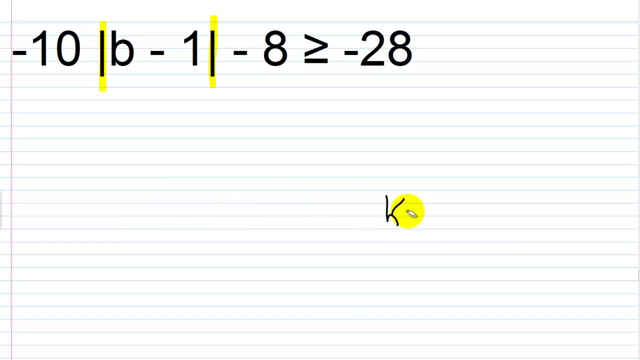 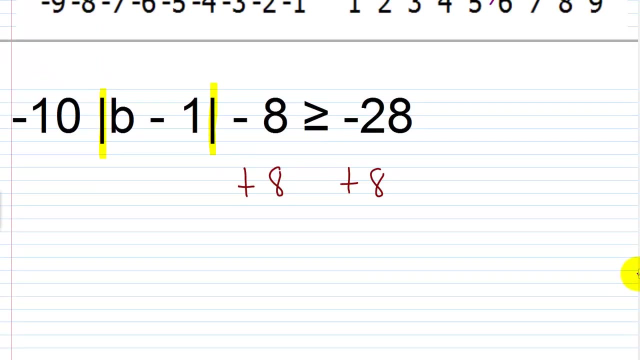 And we want some number on the other side. So to do that, what we need to do Is add 8 to both sides to start. Okay, so this is going to cancel with this, And negative 28 plus 8 is negative 20.. 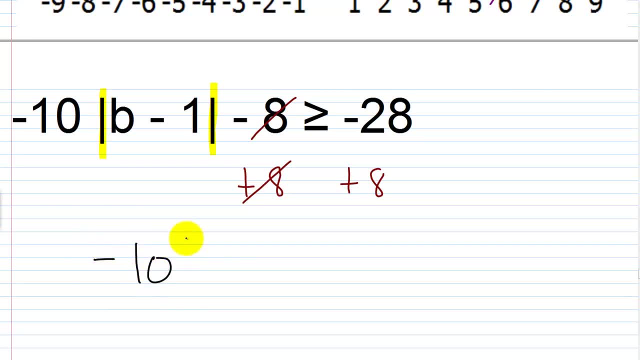 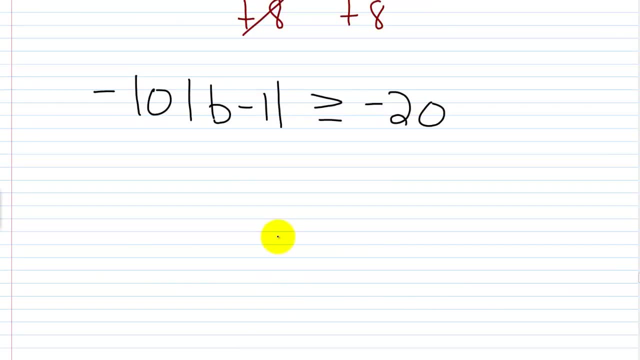 So what I'll have is negative 10 times the absolute value of b minus 1. Is greater than or equal to negative 20.. So now what I want to do is divide each side by negative 10.. Alright, that's what's multiplying this absolute value operation over here. 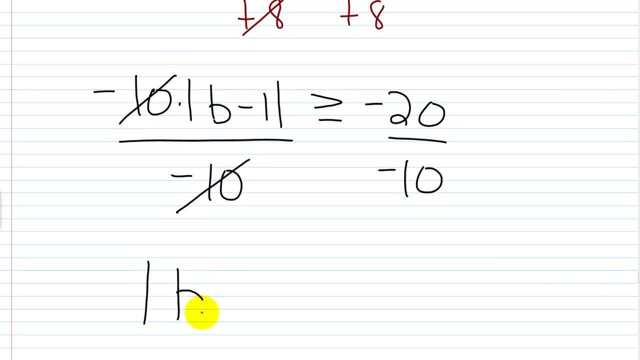 And so this would cancel. with this, I'd have the absolute value of b minus 1.. This would flip Right. we divided by a negative, So this would become less than or equal to, And then negative 20 divided by negative 10 is 2.. 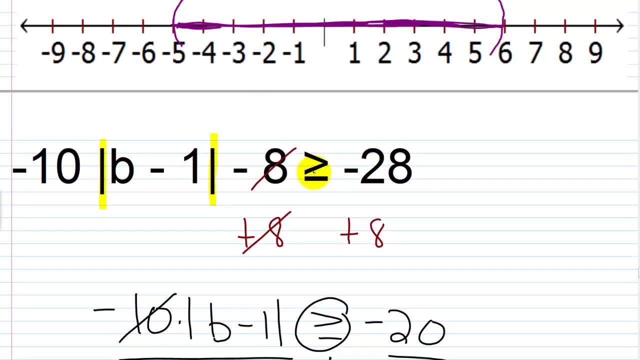 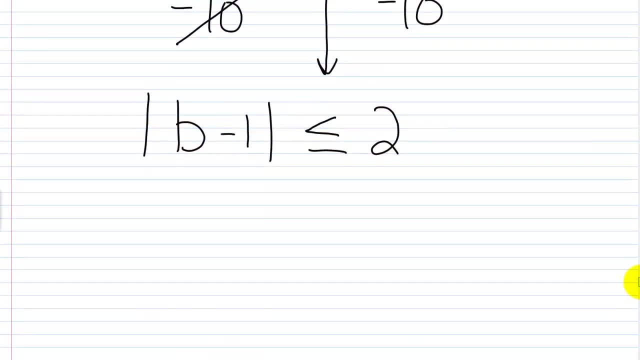 So one thing I want to note is that we started out with this kind of greater than symbol. I know it's a greater than or equal to symbol, But it's a greater than symbol. So we were thinking: or Alright, when you see greater than you're thinking, or. 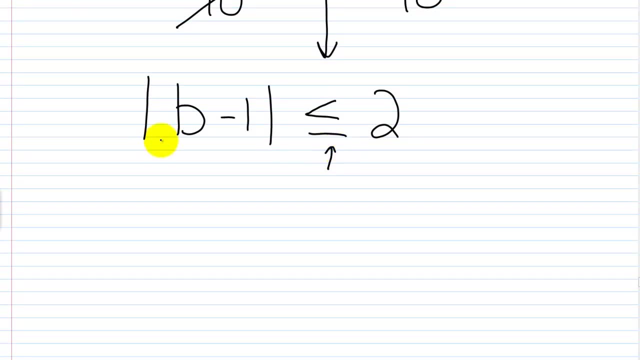 Now, once we went through and we isolated Right, we have our absolute value operation on one side, Number on the other. We see that we have a less than So. we're thinking and Okay, So the first setup is to just remove the bars. 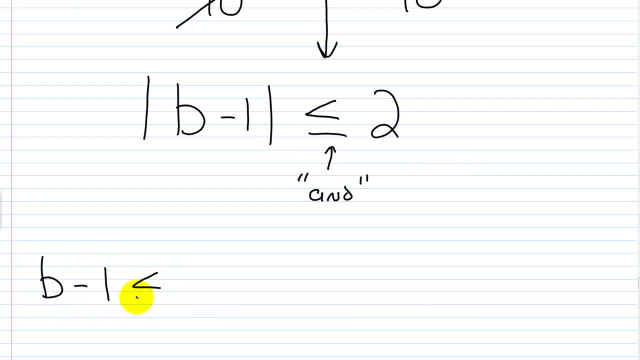 And write what you see. So b minus 1 is less than or equal to 2.. That's your first scenario, Then, and Your second scenario: Remove your bars. So b minus 1.. Flip the sign. So now this is greater than or equal to. 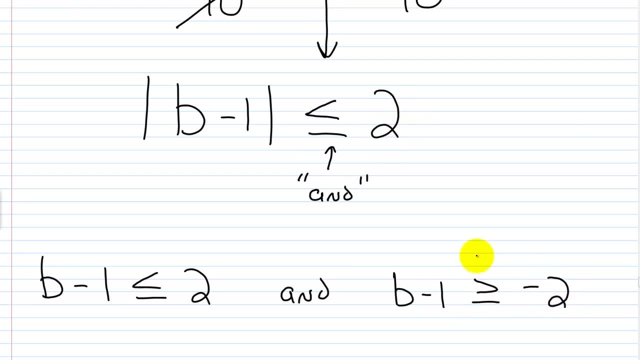 Make this negative, So this would become negative 2.. So let me just write this again. I'll keep writing it: Flip Make negative, Just so you remember. And we can easily just write this as a 3 part inequality. So b minus 1 is in the middle. 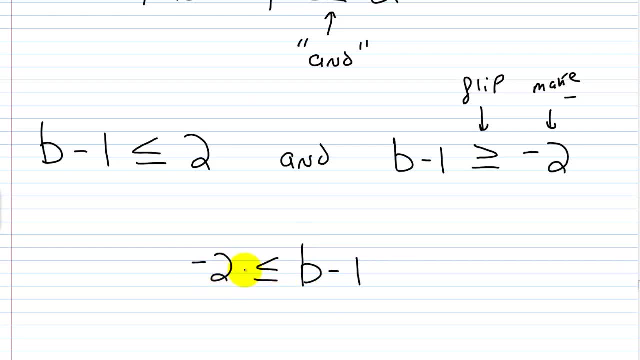 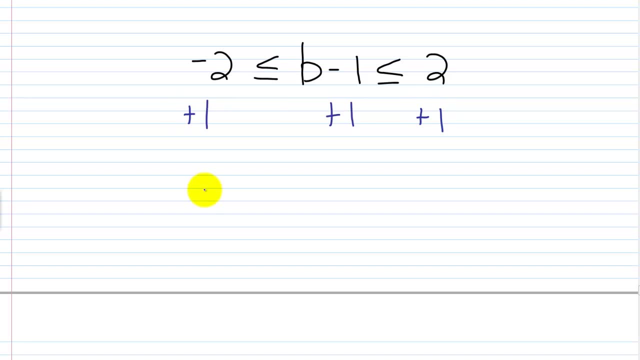 And it's greater than or equal to negative. 2.. And it's less than or equal to 2.. So, to solve this, let's start by adding 1 to each part, And this will be negative. 1 is less than or equal to b. 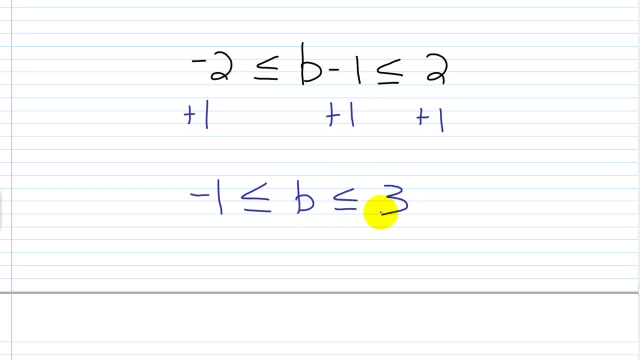 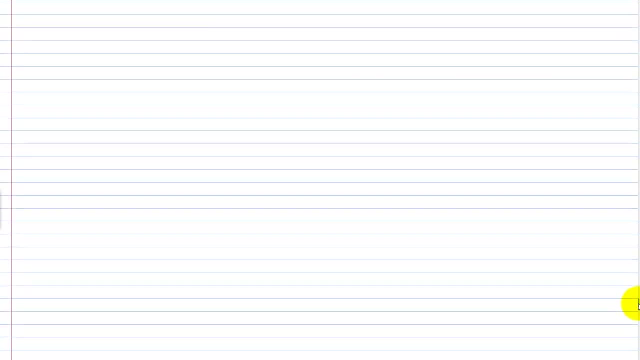 Which is less than or equal to 3.. So basically, b can be any number Between negative 1 and 3. Including both negative 1 and 3. Let's kind of come down here and write that. So again, b is greater than or equal to negative 1.. 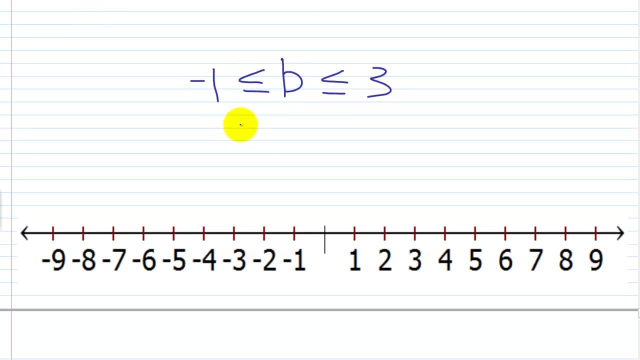 And less than or equal to 3.. So in interval notation It includes both negative 1 and 3.. So we're going to use a bracket in each case And then, graphically, I'll put a bracket at negative 1.. 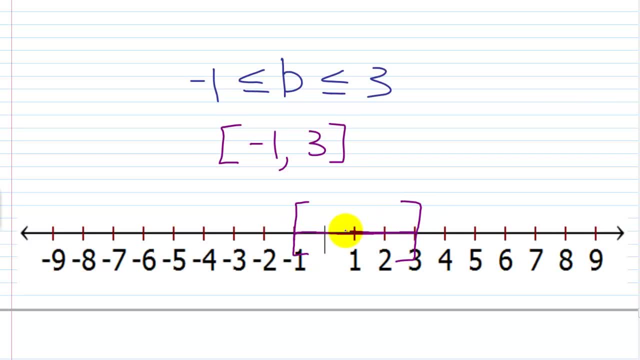 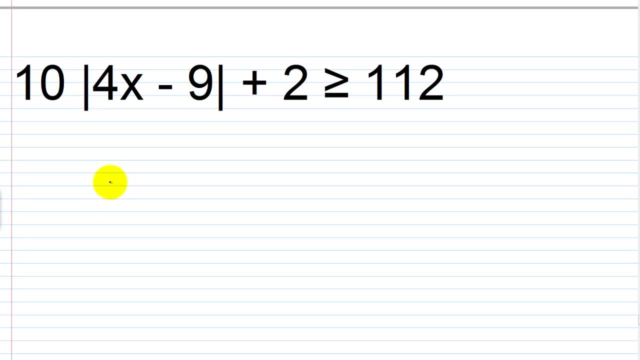 I'll put a bracket at 3.. And then I'll just shade everything in between. Okay, let's take a look at one more like this: So we have 10 times the absolute value of 4x minus 9.. Then plus 2 is greater than or equal to 112.. 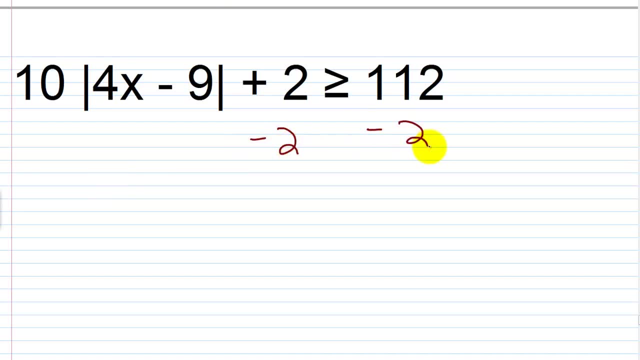 So let's subtract 2 away from each side to start. That's going to cancel. Then we're going to have 10 times the absolute value of 4x minus 9.. Is greater than or equal to 110.. Now to get this absolute value operation. 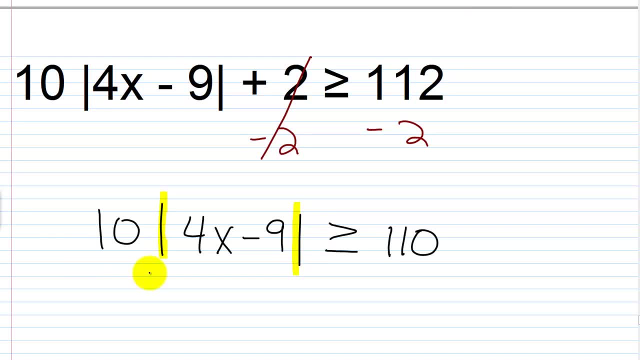 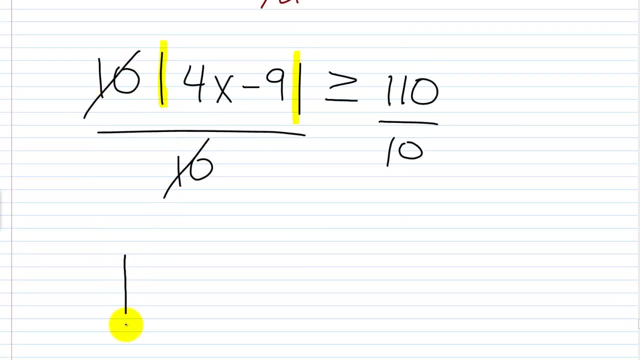 By itself on one side, I still need to divide both sides by 10.. Alright, that's what's multiplying. Divide by 10. over there, This 10 will cancel with this 10.. So I'll have the absolute value of 4x minus 9.. 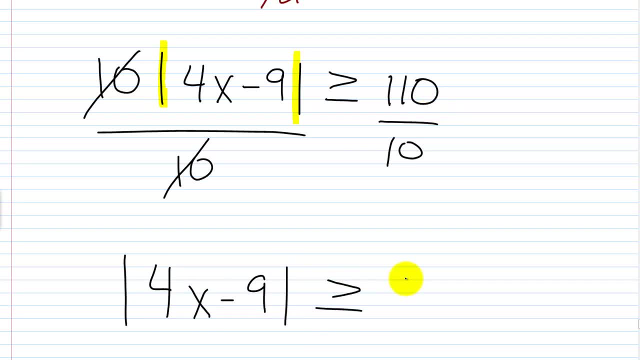 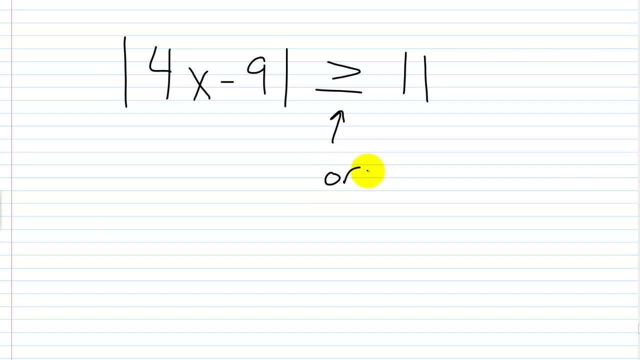 Is greater than or equal to. 110 divided by 10 is 11.. And so now we're ready to apply our rule. We know that this is going to be an or statement, Because it's a greater than. I know it's a greater than or equal to. 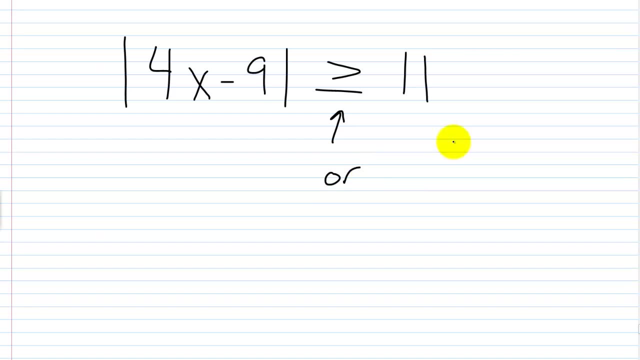 But it's greater than we think about, or So remove the bars to start. So 4x minus 9. Is greater than, or equal to 11. Or Okay, or Then remove the bars, So 4x minus 9.. 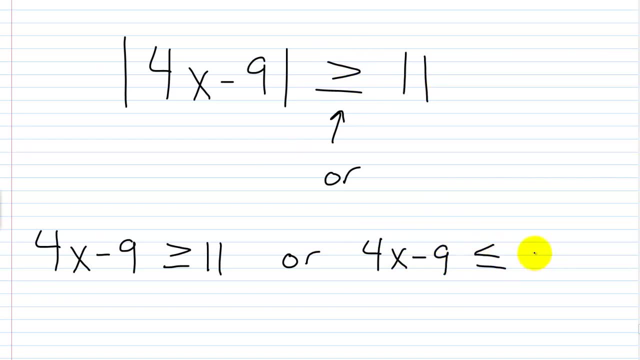 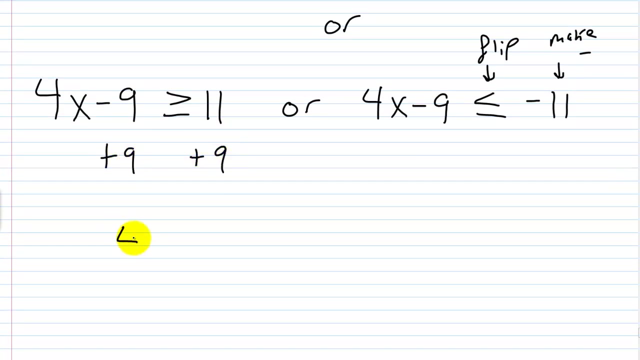 Flip the sign. So flip the sign. Make this negative, Negative. 11. Flip Again: make negative. Alright, So let's solve these two. For this one, I'm just going to add 9 to each side to start, And I'll get 4x is greater than or equal to 20.. 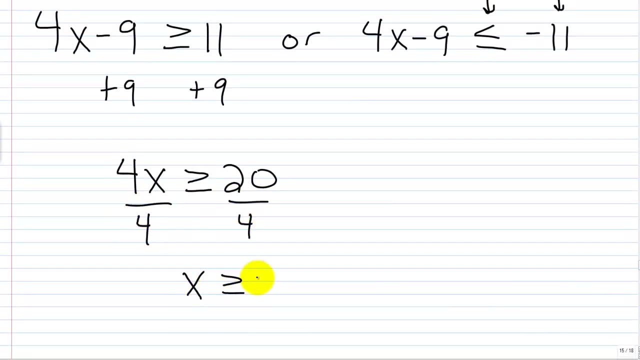 Divide each side by 4. And we get x is greater than or equal to 5.. Over here, if I add 9 to each side, I'll get 4x is less than or equal to negative. 2.. Divide each side by 4.. 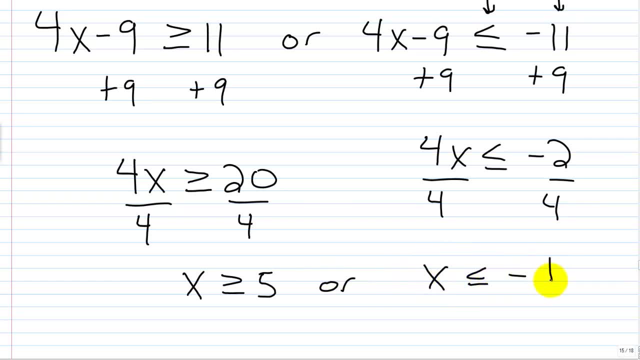 And we're going to get. x is less than or equal to negative 1 half, So x is greater than or equal to 5.. Or x is less than or equal to Negative 1 half, So let's scroll down Again. x can be less than or equal to negative 1 half. 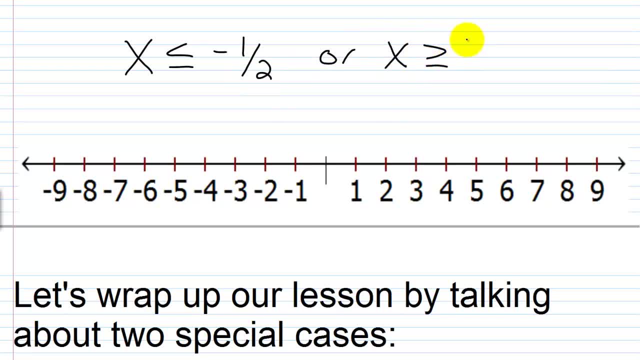 Or x can be greater than or equal to The number 5.. So in interval notation we'll use the union of these two sets. So this one: We'll have a negative infinity here Up to and including negative 1 half. 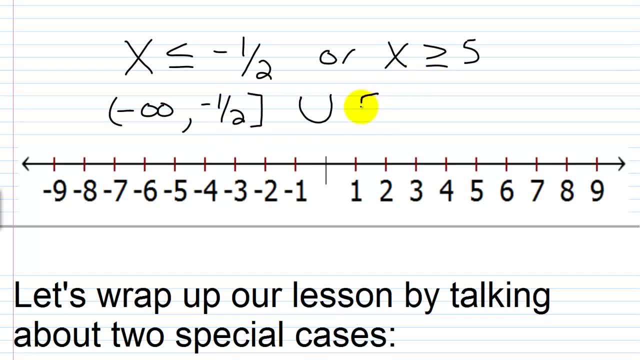 Then the union of that with this other set. It includes 5. So we'll put a bracket there And it's anything larger, So it goes out to infinity. Now, graphically, Kind of look at this one here first. We'll look at negative 1 half. 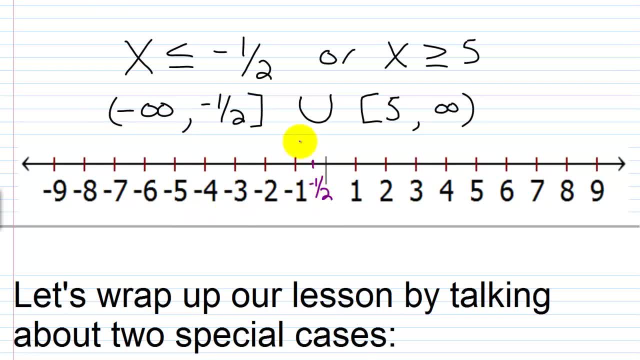 Let's say that's about right there, Negative 1 half. We'll put a bracket there And then we'll shade everything to the left, Everything to the left, And then for this one we'll start at 5.. And we'll put a bracket at 5 because it's included. 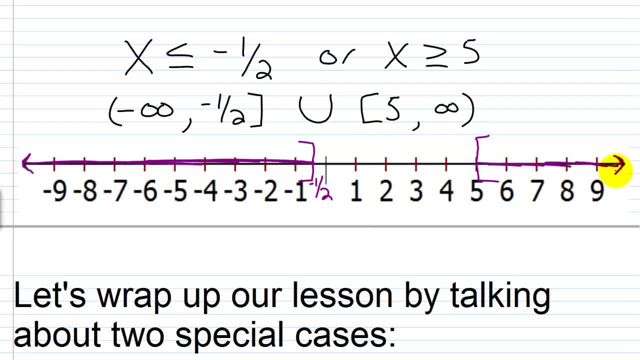 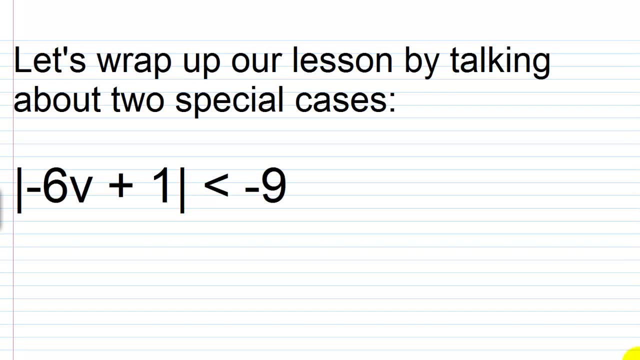 And we'll shade everything to the right. So this would be your solution, set graphically Okay. So what I want to do now Is just wrap up our lesson by talking about two special cases, And no doubt these will be on your test. 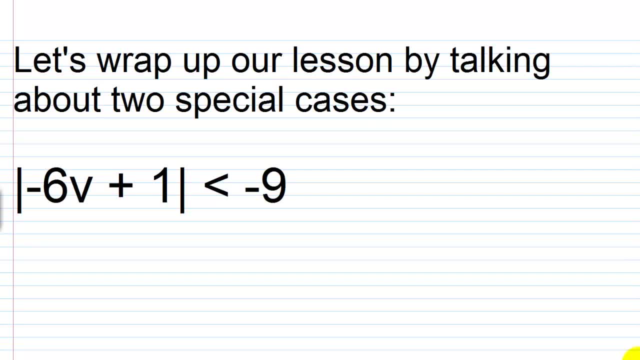 If you take a test on absolute value inequalities, Your teacher will give these to you. So we start with the absolute value of negative. 6v plus 1. Is less than negative 9.. So a lot of people see this And they just go right into it. 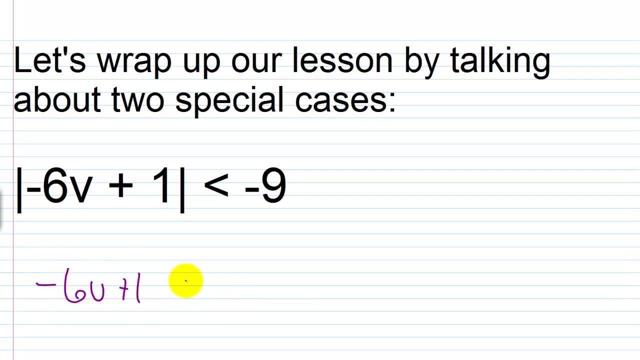 They go: okay, Well, negative 6v plus 1 is less than negative 9.. And then this is a less than. So we'll say: and You know, negative 6v plus 1 is flip the sign And then make this into a positive 9.. 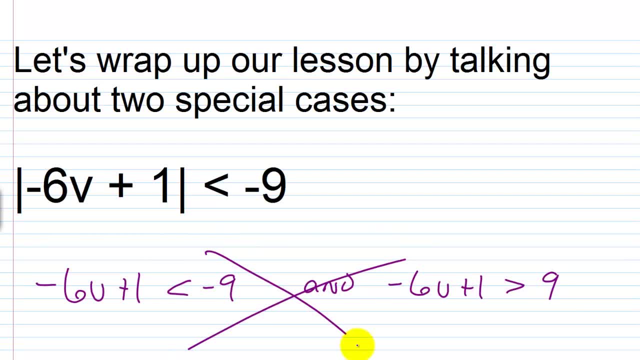 That's wrong. The reason is you just have to stop and think about what absolute value means for a second. The absolute value of a number is a distance. It's never going to be negative. You can say the absolute value of x is greater than or equal to 0.. 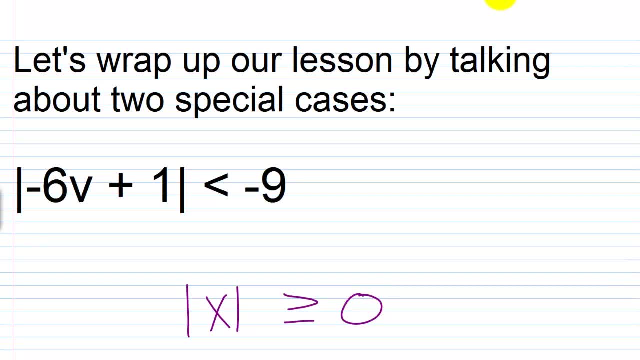 It can be 0 or anything greater. So this right here, The fact that it says the absolute value of this is going to be less than a negative, It's not possible. If it's negative, You take the absolute value of it. 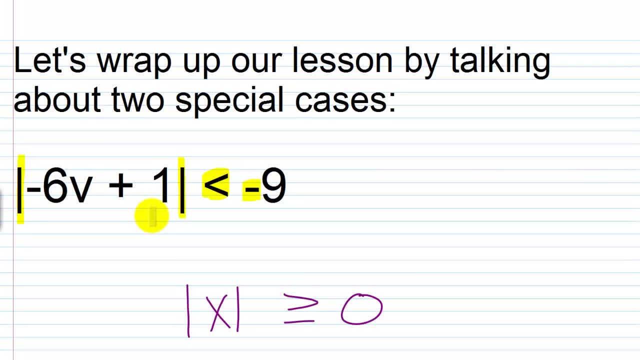 It becomes positive. And if it's 0. It's going to be 0. None of those scenarios will ever, ever, ever result in it being less than negative 9. It can be 0 or anything greater. So this right here. 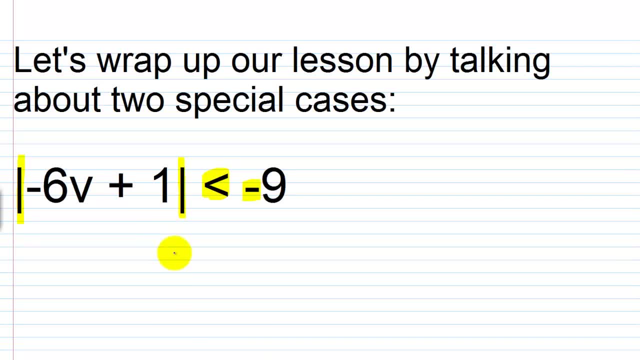 When you see something like this: There's no solution. There's no solution, So you could write that. Or typically you'll see this symbol drawn. It means that your solution set contains no elements, So you can write this or that, But you don't have a solution here. 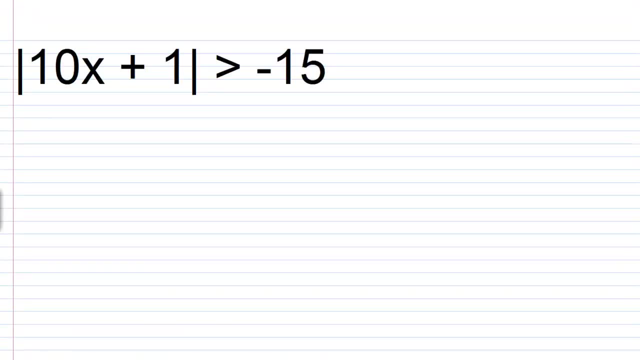 Alright, Let's look at the other scenario that you're going to get And in this scenario you have the absolute value of 10x plus 1 is greater than negative 15.. Well, again, Think about what absolute value means, The absolute value of this. 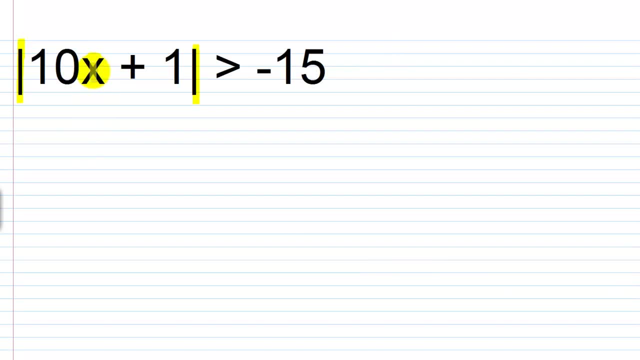 Okay, Whatever it is, I'm going to take some number, Plug it in for x, I'm going to multiply it by 10. Add 1 to it And then I'm going to perform this absolute value operation. If this is negative. 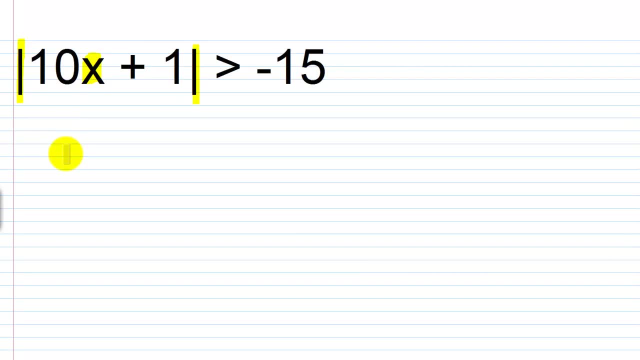 Okay, If the result of this is negative, Then I take the absolute value of it. I'm going to get a positive number. Any positive number is always greater than negative 15.. If it's 0. That's greater than negative 15.. 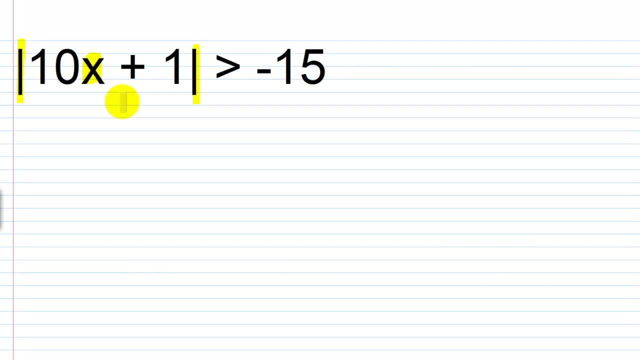 And if it's positive, Take the absolute value of it. It's just still positive. That's greater than negative 15. So no matter what I plug in for x here, It won't matter, It'll always be true. This will always be true for any real number.